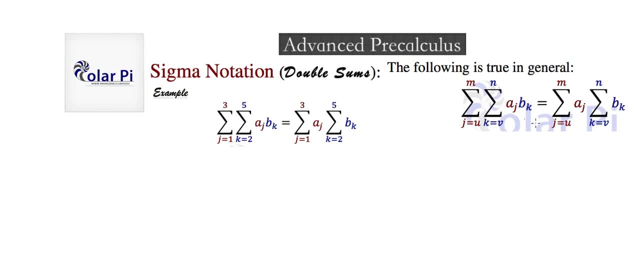 side By this property here we know that it would equal this right-hand side here right. So to demonstrate that this is true, let's first work with the left-hand side. So when we work with the left-hand side, since we have a double sum, 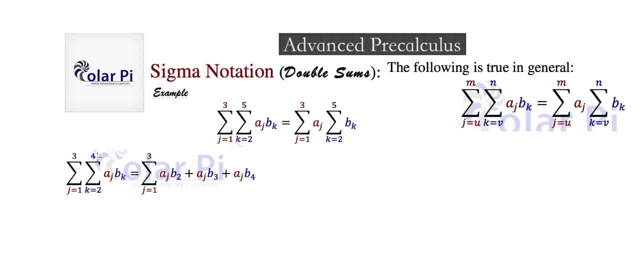 we need to first take care of the inner sigma. So the sigma inside and the sigma inside involves the b sub k's right. So taking care of that first, we see that we have to leave the a sub j's alone, because this k index does not involve the a sub j's at all. It only involves the b sub k's. So 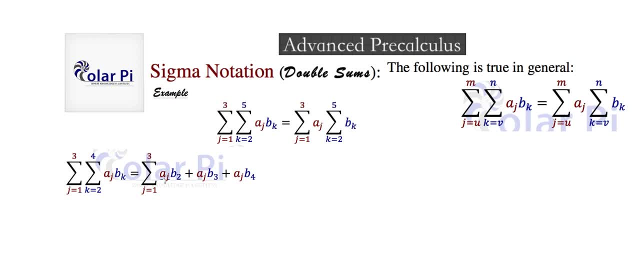 taking care of the b sub k's. we have j equals 1 to 3 of a sub j times b sub 2, because we start with k equals 3.. So we have a sub j times b sub 2, because we start with k equals 3.. So we have a. 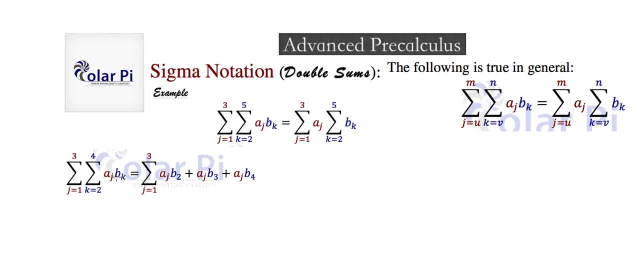 sub j, times b, sub 2, so there, and then plus a sub j, and then times b, sub 3 is next, and finally a sub j and b sub 4 is last. right, Okay, cool, cool, cool. So now here, all we have to take care of is the a. 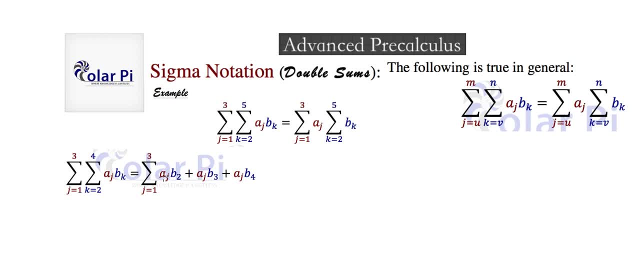 sub. j's starting with j equals 1.. So when j equals 1, we'll have a1 b2 plus a1 b3 plus a1 b4. And then we'll have plus when j is 2, we'll have a2 b2 plus a2 b3 plus a2 b4. So we have a1 b2 plus a2 b3. 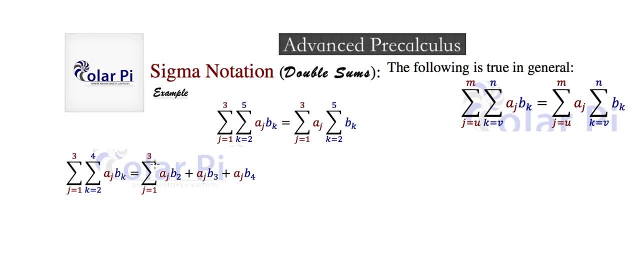 plus a2 b4.. Plus, finally, when j is 3, I will have a3 b2 plus a3 b3 plus a3 b4. And so that would be this, On the other hand, if we worked with this right-hand side instead, we know that the right-hand 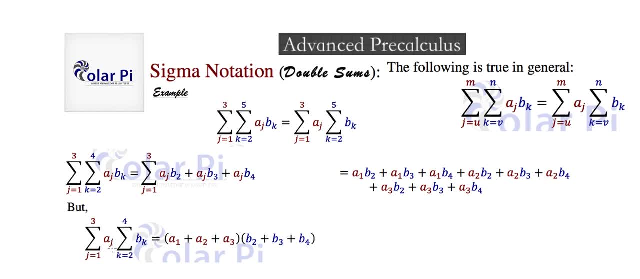 side here, which is this: here is the same thing as taking care of this sigma, taking care of that sigma and then multiplying them together. But taking care of this sigma just means adding a1,, a2, and a3. And taking care of this sigma means adding b2, b3, and b4. And when we multiply, 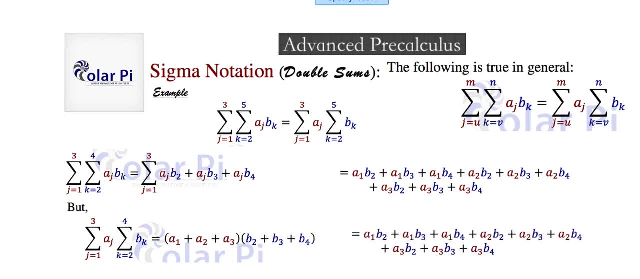 this here. unsurprisingly, we get this, which is the same as what we had had, And therefore, at least with this example, we've demonstrated this property. This is not a proof, but it's a demonstration that this property works. yeah, Okay, cool, cool, All right. so the next video.